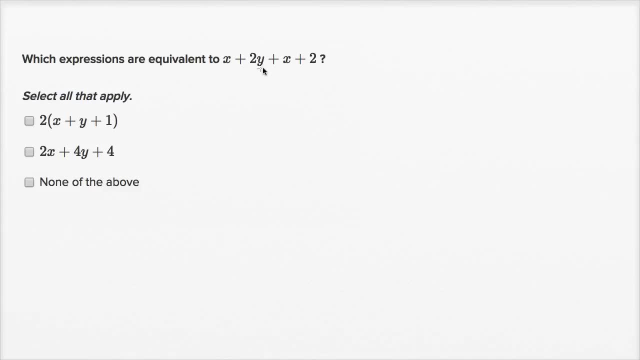 Which expressions are equivalent to x plus 2y plus x plus 2?? Select all that apply. All right, let's see if I can manipulate this thing a little bit. Let me just rewrite it: So I have x plus 2y plus x plus 2.. 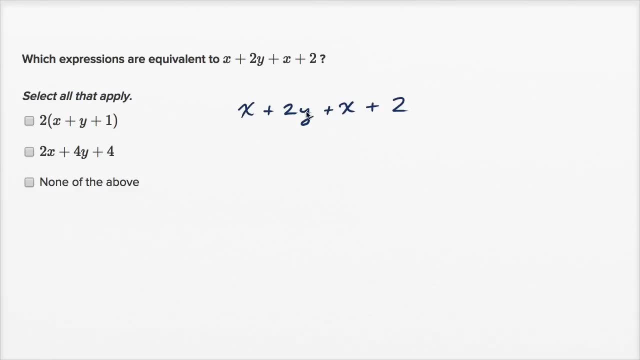 So the first thing that jumps out at me before I even look at these choices: here I have an x over here, I have an x over there. Well, if I have one x and then I can add it to another x, that would be 2x. 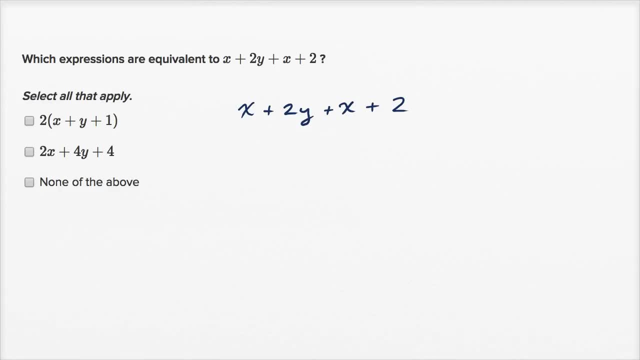 So I could rewrite this. let me do this in a different color. I could rewrite this x and this x. if I add them together, that's going to be 2x. So this is actually. I don't want to skip any steps. 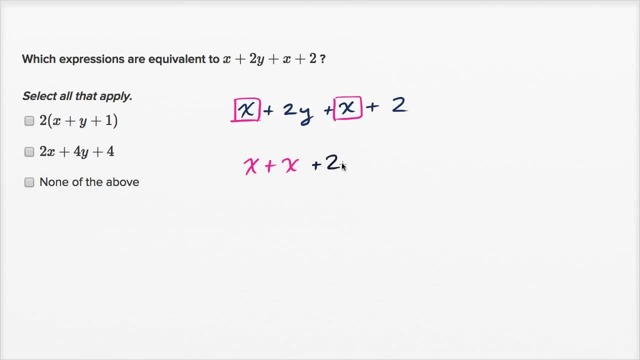 So that's x plus x plus 2y. now I'm just switching the order plus 2, and then these two x's right over here. I could just rewrite that as 2x, So I have 2x plus 2y plus 2y plus 2x. 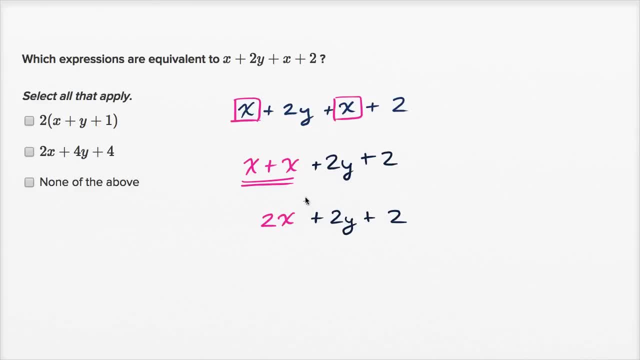 Now let's see out of all of my choices, so this one: this is 2x plus 4y plus 4.. So that's not right. I have 2x plus 2y plus 2, so I can rule this one out. 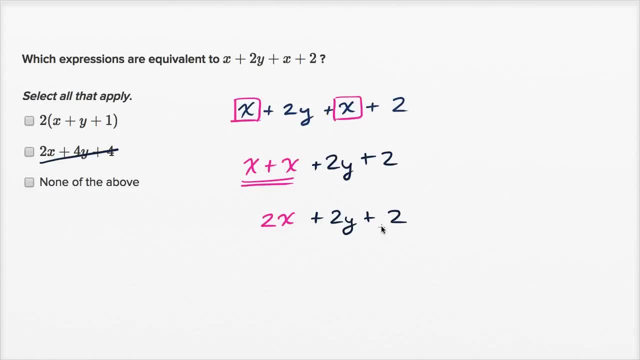 Now this one's interesting. it looks like they have factored out a 2, let's see, if we factor out a 2 here, what happens. So we do see that 2 is a factor of that term, it's a factor of that term and it's a factor of that term. 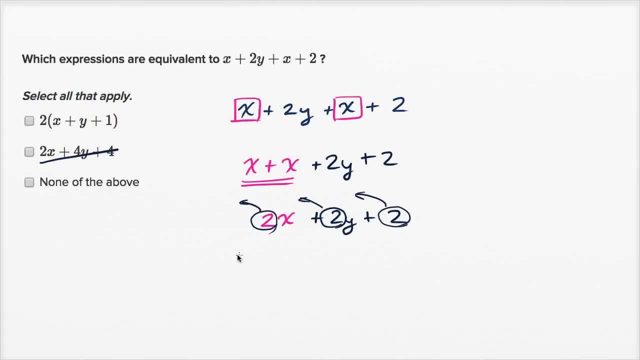 so let's see if we can factor it out. So this is going to be two times x. I'll do the x in that same magenta color. two times x plus, you have just a y left when you factor out the two. 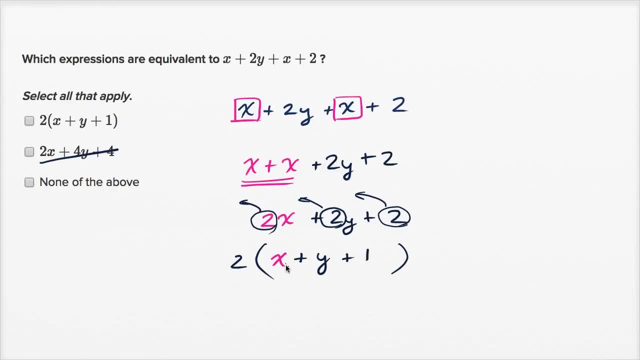 and then if you factor out a two here, you're just gonna have a one left. So two times x plus y plus one, which is exactly what they have over here, And since I was able to find a choice, I will not pick none of the above.